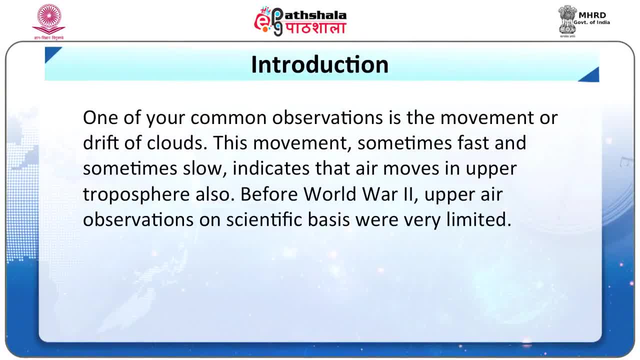 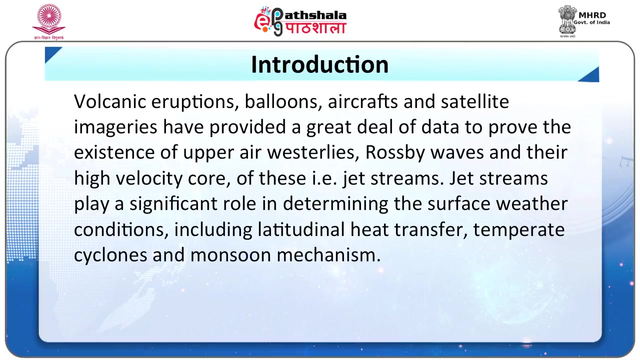 6. You will be able to describe the Volcanic eruptions balloons. aircrafts and satellite imageries have provided a great deal of data to prove the existence of upper air westerlies, Rossby waves and their high-velocity core ie jet streams. 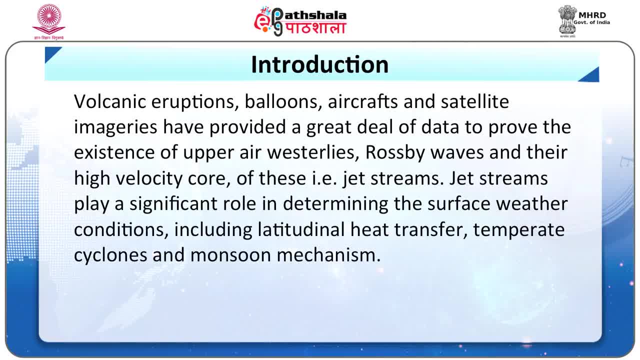 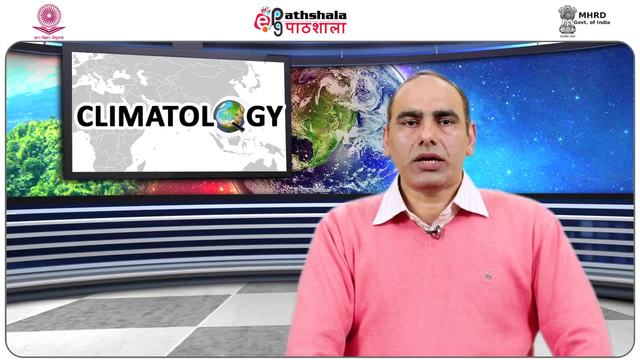 Jet streams play a significant role in determining the surface weather conditions, including latitudinal heat transfer, temperate cyclones and monsoon mechanism. In this module, our focus is on the understanding of upper air circulations and especially jet streams. Temperature, atmospheric pressure and air circulations are quite different in upper part of the world. 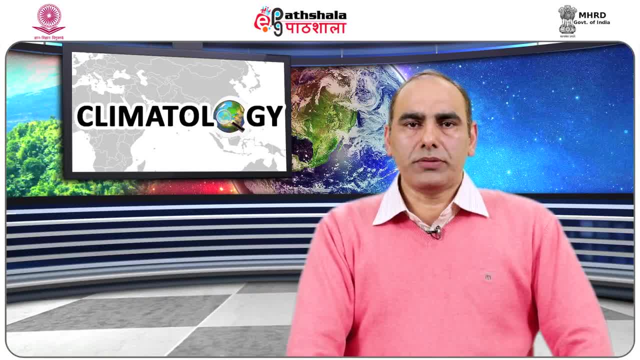 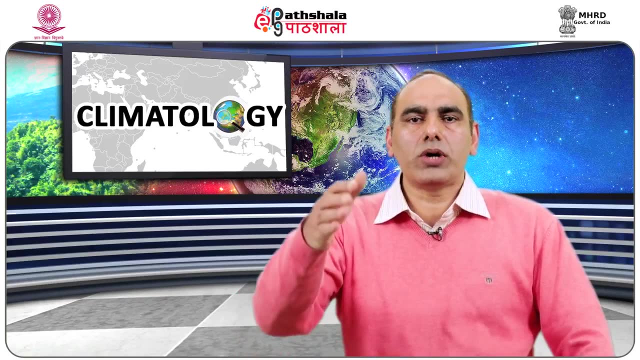 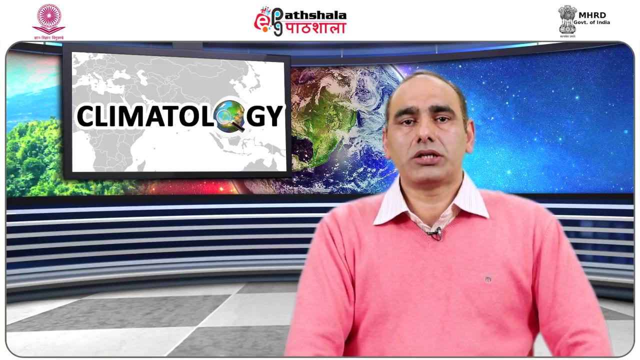 As compared with those prevailing near the Earth's surface. the upper air circulations are predominantly geostrophic. Recall that pressure gradient force, which is always perpendicular to isobars, onsets motion of partial of air from high-pressure area to low-pressure area. 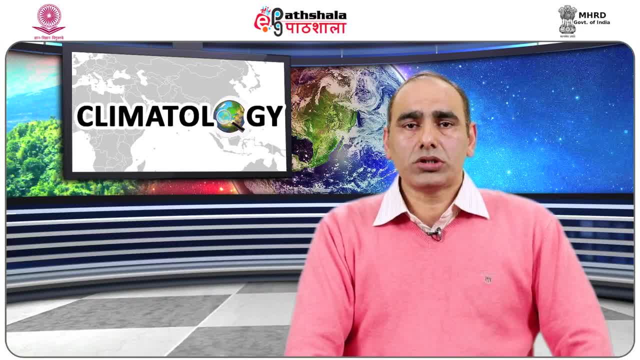 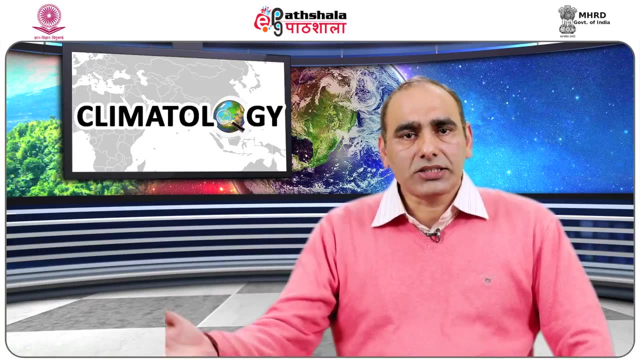 You also have idea from previous modules on planetary pressure. In this module we will discuss about atmospheric pressure, pressure belts and general atmospheric circulation that, as winds start blowing, due to rotation of Earth, Coriolis force deflects it towards right-hand side in the northern hemisphere and its magnitude is proportional to wind speed. 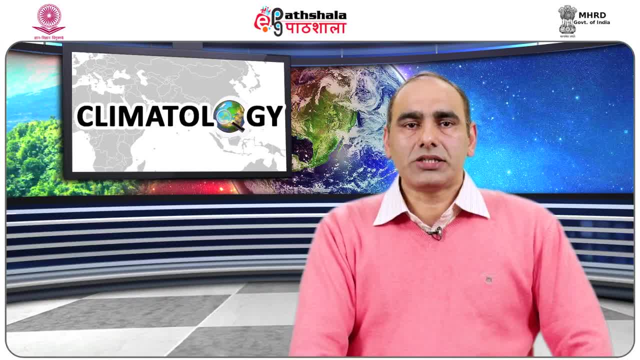 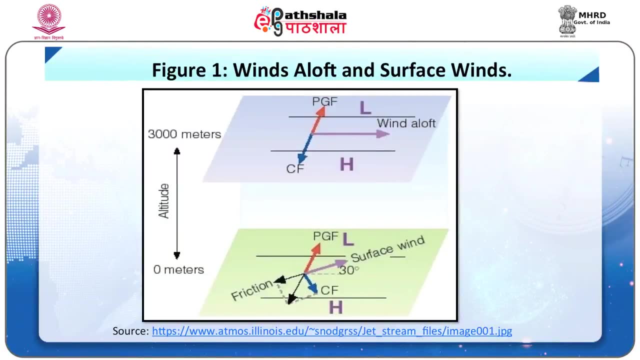 Therefore, as the partial of air accelerates, its deflection increases. Finally, a situation comes when wind turns, So much so that it starts blowing parallel to the isobars. This represents the situation of the geostrophic balance, that is, two opposing forces. pressure, gradient force and Coriolis force are exactly same. Therefore, the resultant winds are known as geostrophic winds, as is shown in figure number 1.. In the middle and higher latitudes of both the hemispheres, upper air westerlies prevail due to balancing act of pressure, gradient force and Coriolis force. 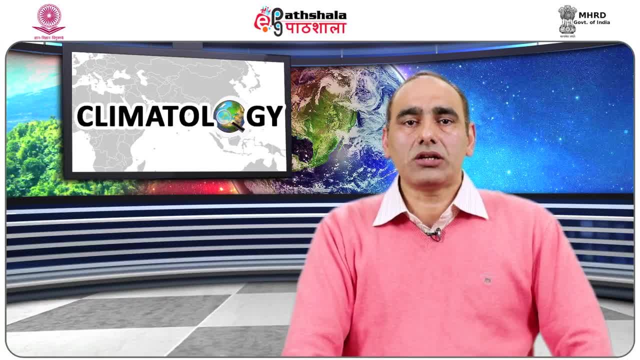 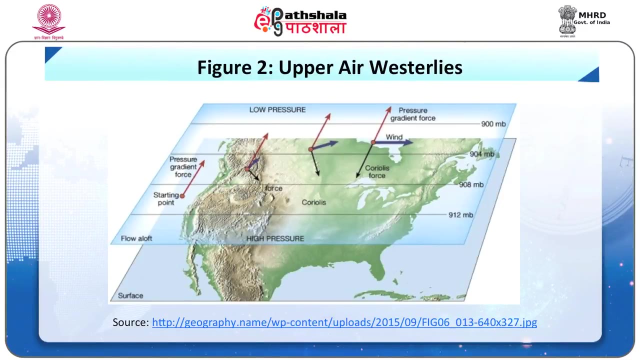 It is well known that winds are result of pressure variations and speed is directly related to pressure gradient. The relationship between pressure and wind direction was first formulated as Bayes-Ballet's law in 1857. It states that if you stand with your back to the wind in the northern hemisphere 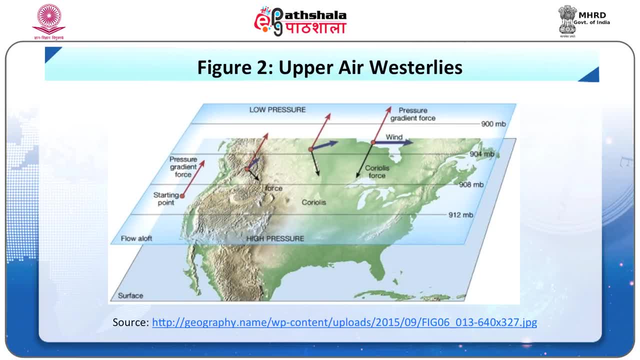 your low pressure will be found to your left and high pressure to your right. You can verify this case of upper air westerlies in figure 2, In the upper part. this is the example of westerlie case shown in figure 3.. 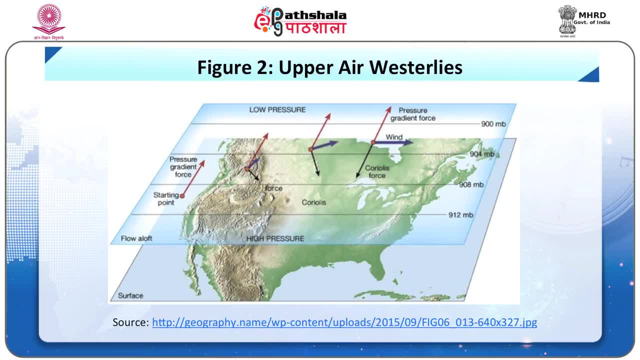 Atmospheric pressure is low towards the pole and high towards equator. It is also noteworthy that in upper air, atmosphere decreases according to which area of the atmosphere is etched. Atmospheric pressure also goes down to the bottom. Atmospheric pressure decreases according to level and temperature of the�合4m Eph SSD. 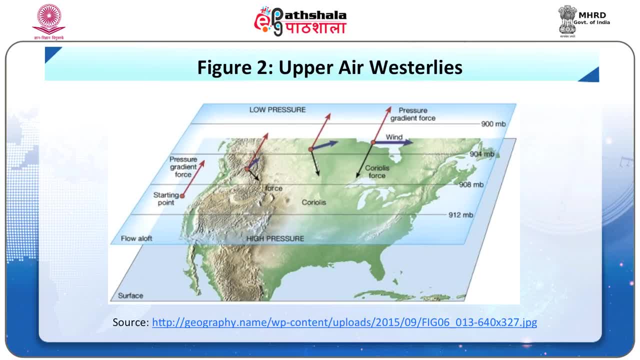 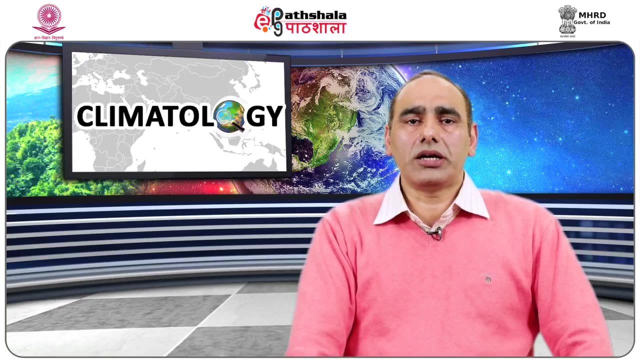 decreases towards poles In upper part. pressure gradient increases with height. Therefore wind's velocity increases with height, But this is generally limited to tropopause. Further, the balancing act of pressure, gradient force and Coriolis force is resulting into the development of upper air westerlies Poleward from the tropical headly circulations in both. 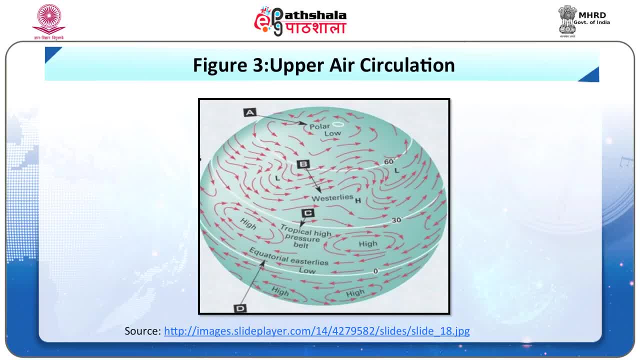 the hemispheres. air flow in the troposphere is normally and persistently west to east, generally parallel to latitudes as upper air westerlies. You can refer figure number 3 for this. The figure 3 shows four major elements of upper air conditions, namely a, Polar, low, b, Persistence. 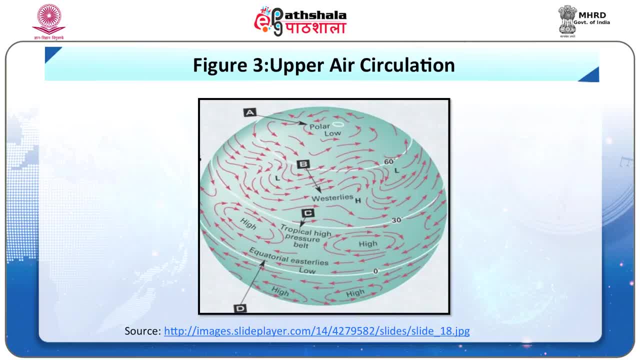 of upper air westerlies in the middle c Tropical high pressure belt, which is constituted by a number of high pressure cells, And b- Equatorial easterlies, between equator and subtropical high pressure cells. The upper gseeustrophic winds are easterly. 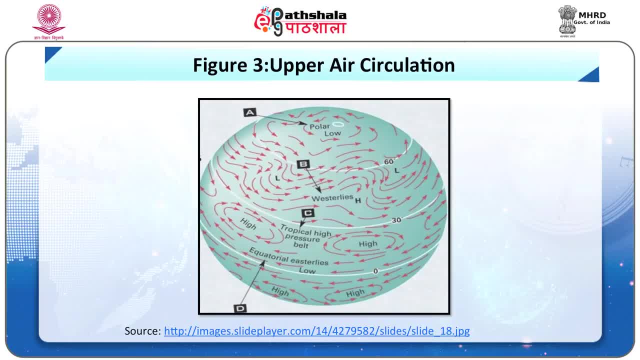 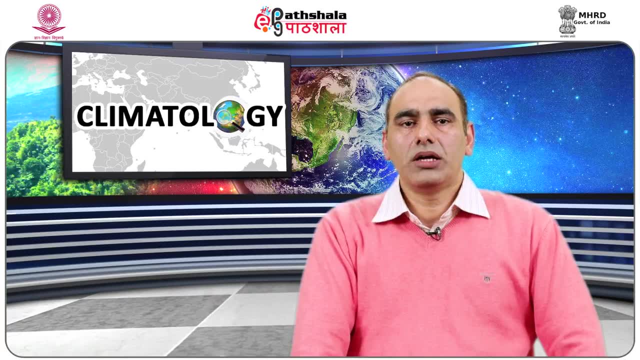 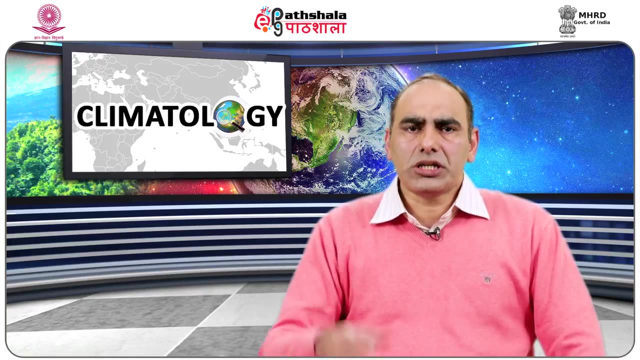 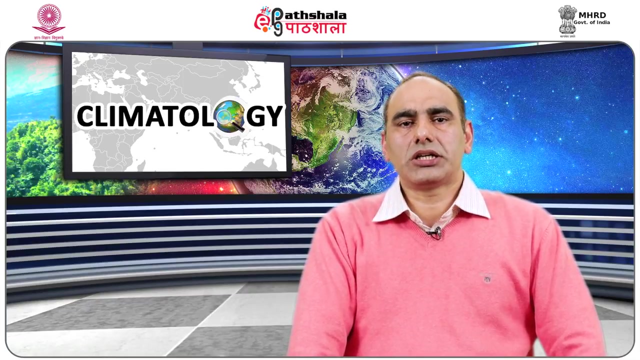 Similarly is the condition in the southern hemisphere. The uniform flow of upper air westerlies is frequently disturbed by the development of śm of large-scale undulations known as Rossby waves. The core part of the Rossby waves, with steepest gradients and presence of maximum speed winds in narrow bends, represents jet. 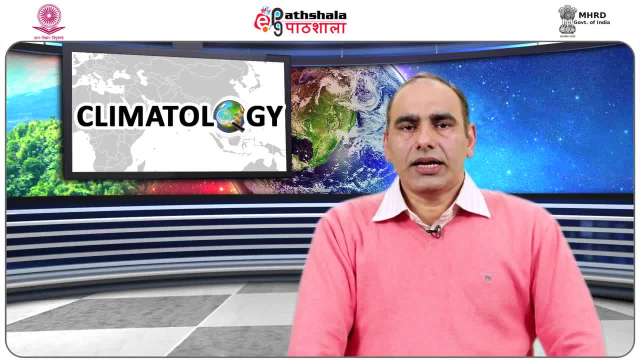 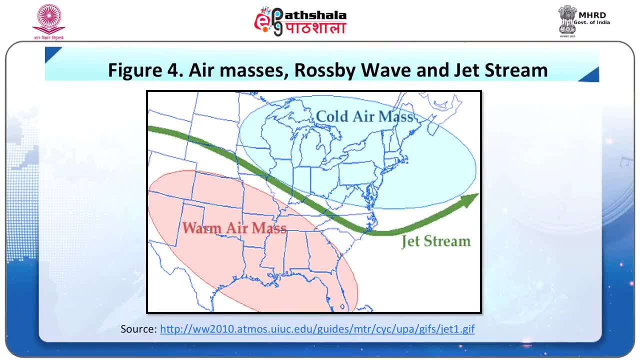 streams, Rossby waves and index cycle of jet streams is our next focus area. The Rossby waves develop along the narrow polar front zone of contact between two contrasting large bodies of air: cold air mass on the poleward side and warm air mass on the equator side. 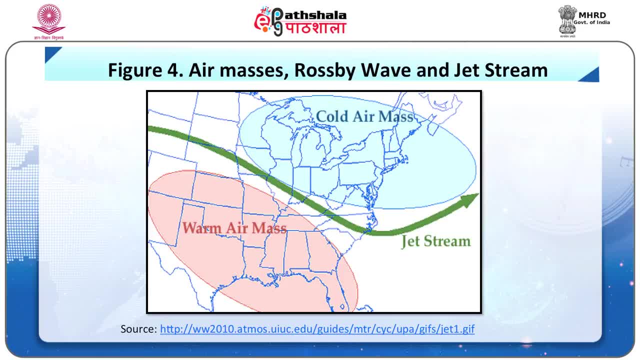 as is shown in figure number 4.. These are called Rossby waves because they were discovered by scholar CJ Rossby in 1937. The direct interaction between their core part of the Rossby waves was experienced by pilots of B-29 jet planes of USA during the World War. 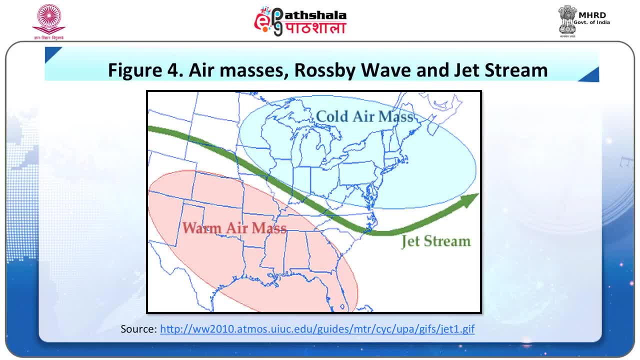 II. The wavelength of the Rossby waves is in the range of 2,000 to 4,000 kilometers on an average. Therefore, about 4 to 6 Rossby waves can be identified around circumpolar region at a time. These waves play a significant role in determining. 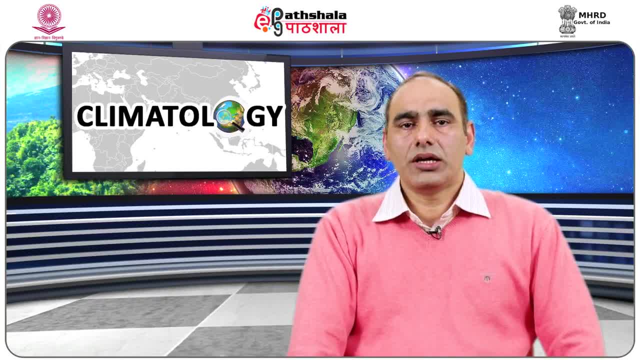 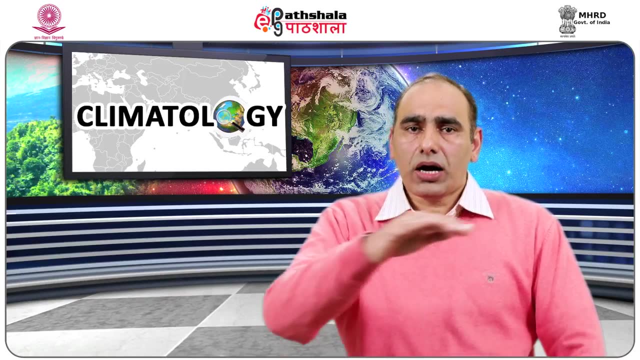 the range of the Rossby waves. The Rossby waves are associated with weather conditions of middle latitudes and are specially associated with genesis of temperate cyclones and anticyclones. The index cycle of jet streams represents the change from straight path to most sinus path of Rossby waves and jet streams. 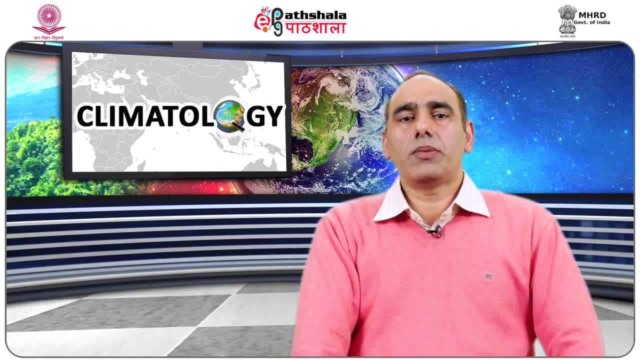 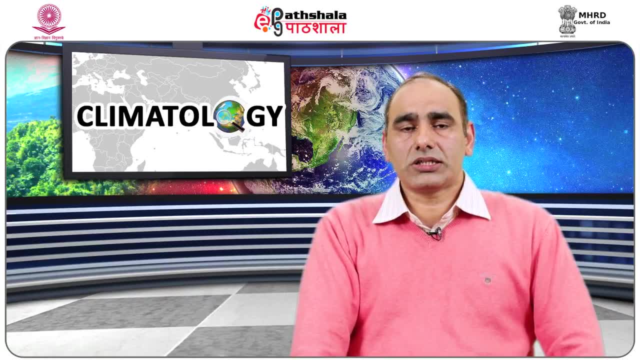 This transformation takes place in about 4 to 6 weeks and is the most common way to determine the range of the Rossby waves. The Rossby waves are usually divided into following four successive stages or phases. We will discuss these phases one by one. 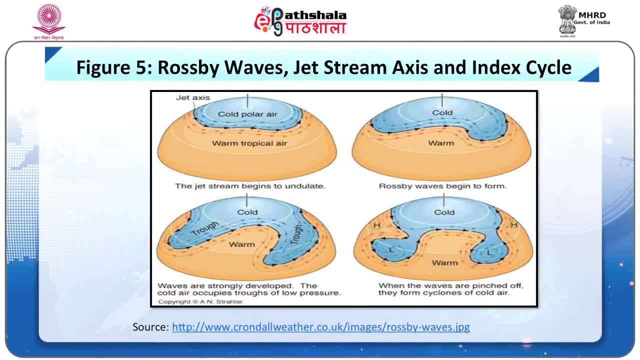 The first stage or phase in this stage, jet stream prevails near the pole and occupies a general east-west direction. It operates in polar front zone with the presence of cold air mass in the north and warm tropical air mass in the south, In the northern hemisphere. 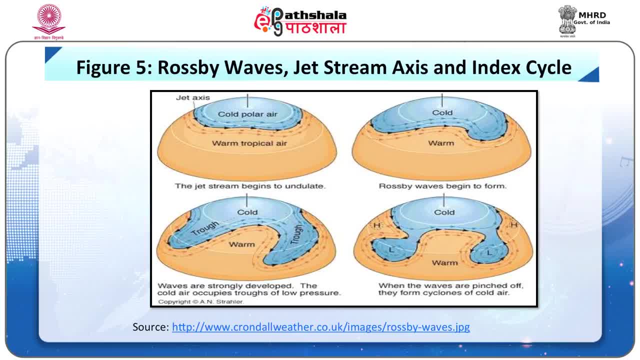 the Rossby waves are fairly smooth and stable and the path of the jet stream is straight, as is represented in figure no 5.. The steep pressure gradient and consequent high-velocity jet streams prevail west to east in this strongly established upper-air-westerly region. The same standard: 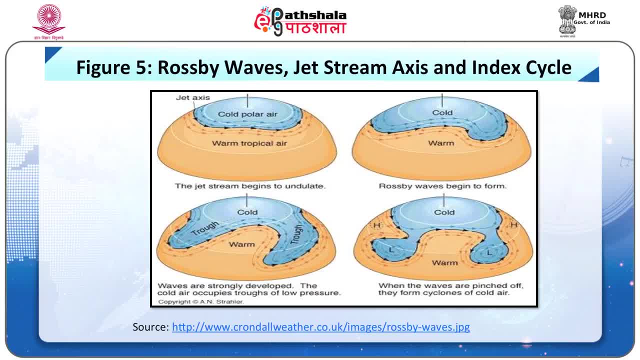 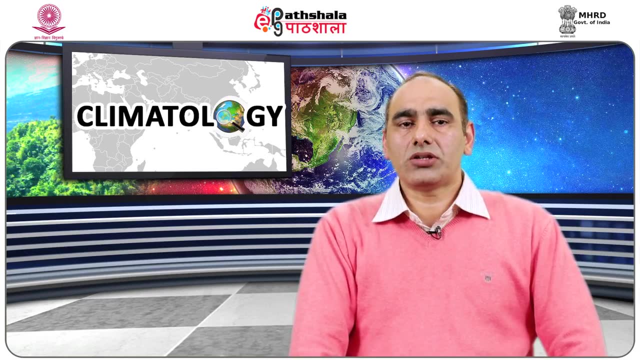 of jet stream animation is used across allPPIs ONLY at the end of the force waves. you In this stage, surface planetary westerlies of mid and high latitudes are strong zonal and located slightly poleward. This stage is known as the stage of high zonal index. 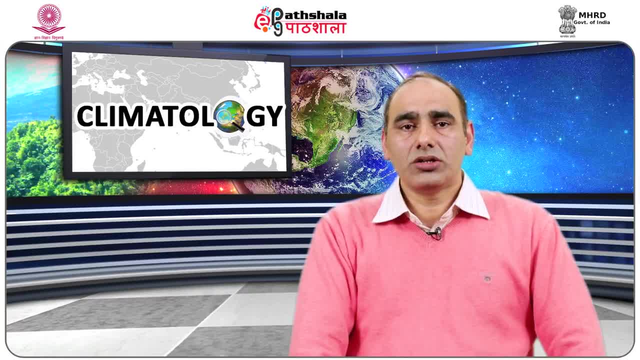 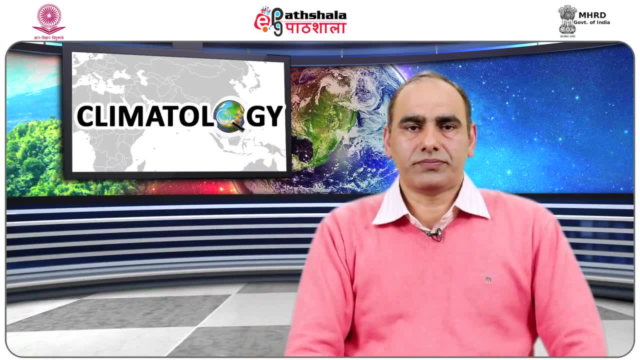 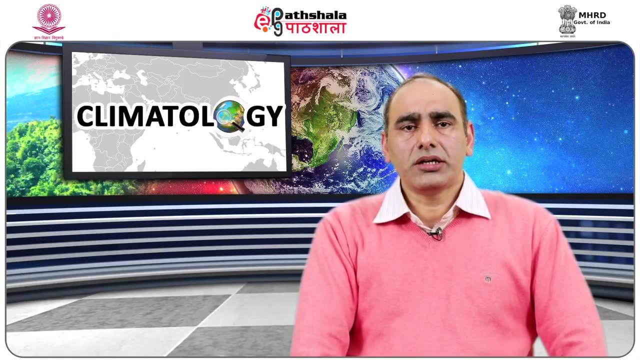 The pressure systems are oriented as zonal, that is, in east-west direction, in particular latitudinal zone. The latitudinal heat exchange is limited and cyclonic activity is prevalent in high latitudes only. Let us come to the second stage. 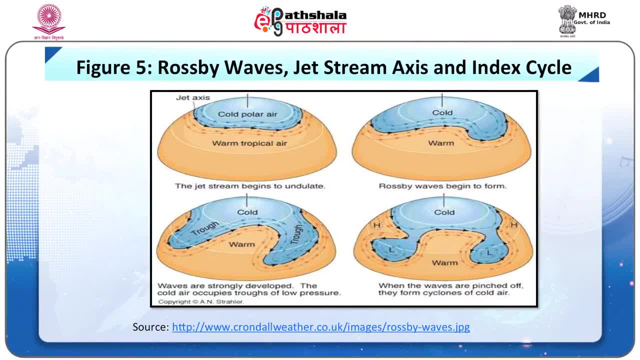 In this stage the straight path of jet stream changes to undulating or wavy path, which means Rossby waves begin to develop. With the passage of time, the amplitude of the jet stream increases And it starts shifting gradually towards equator. 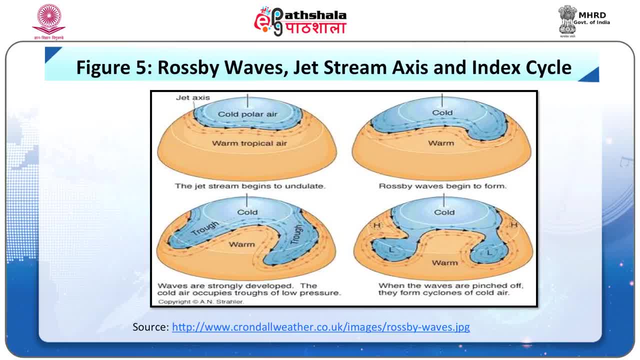 The minor undulations deepen gradually, The cold air makes inroads towards the equator and warm air towards high latitudes. Let us come to the third stage. In this stage, the path of jet stream becomes meandering And its amplitude registers significant increase. 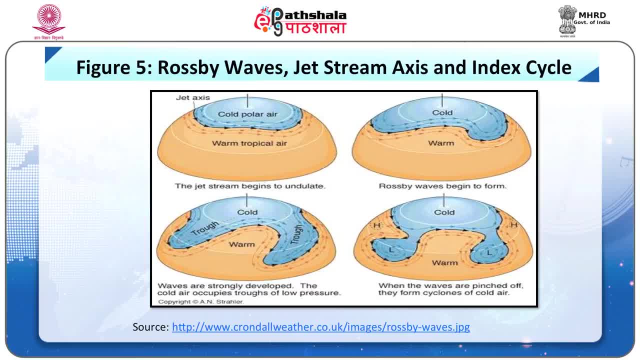 Rossby waves and jet stream moves towards equator and operate up to 20 degree latitudes. The pressure gradient, which was equatorward to poleward in previous two stages, becomes west to east in this stage And large-scale latitudinal heat exchanges occur due to the movement of cold air masses towards equator. 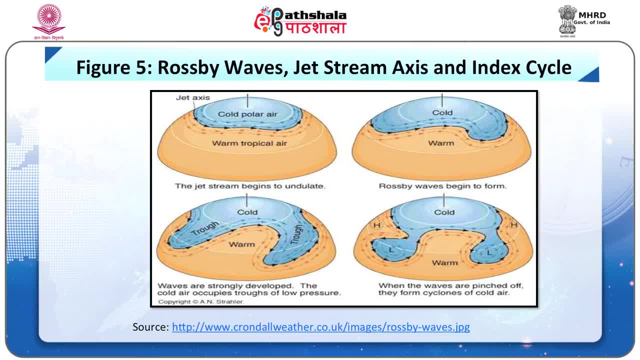 and warm air masses towards poles. The cold air makes inroads into lower latitudes, in deep embayments, which emerge as troughs of low pressure at high levels. Two such troughs of low pressure are clearly visible in the third diagram of figure 5.. 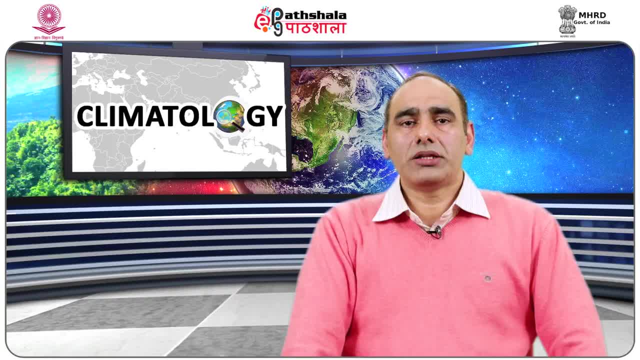 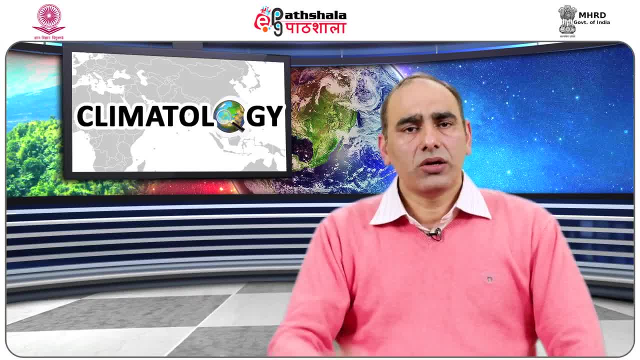 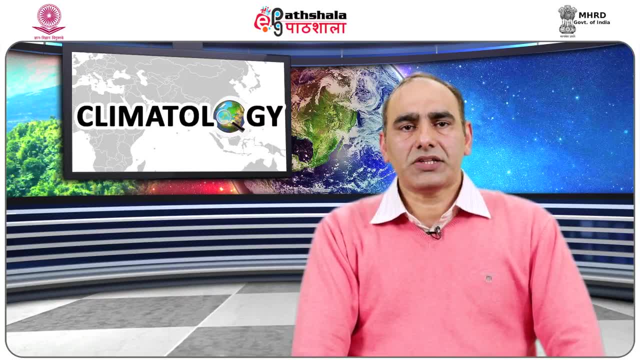 prevails and cyclonic activities on surface are very limited. Conversely, when the aloft air flow manifests large amplitude or curved path having shorter wavelengths, atmospheric instability prevails and is reflected in cyclonic disturbances. Let us come to jet streams, their definition and characteristics. 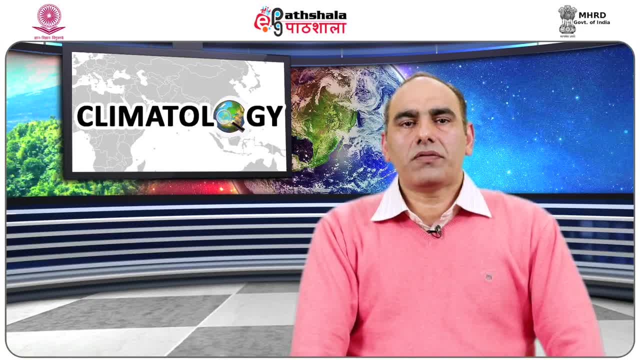 Associated with the Rossby waves is a narrow band of very strong winds known as jet streams. Jet streams are found in mid-latitude upper troposphere, usually blowing west to east, that is, as westerlies. These winds attain their highest values from the west to east. 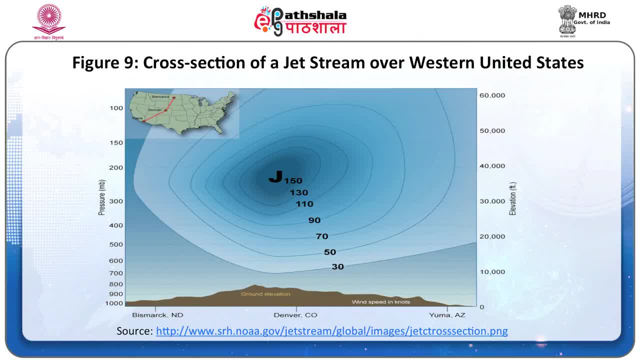 velocities. at 10 to 12 km altitude, the wind velocity is highest at the center and decreases outwards towards its peripheral parts, as can be seen in figure number 9.. This way, it resembles a stream of water moving in a water container. 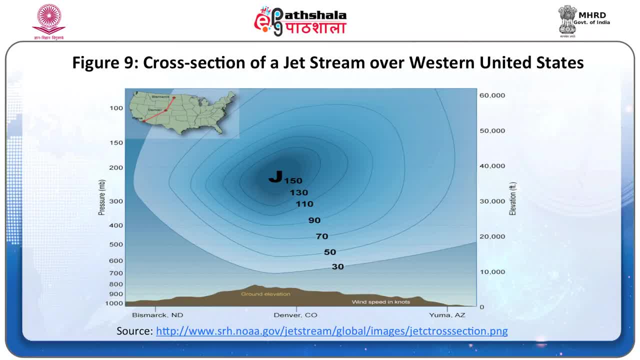 In this figure, number 9,, the cross section of the jet stream shows circular isotechs over western United Streets. Isotechs are line joining places of equal wind velocity. The core, at the height of about 11 km, has the strongest winds, at 150 knots or about. 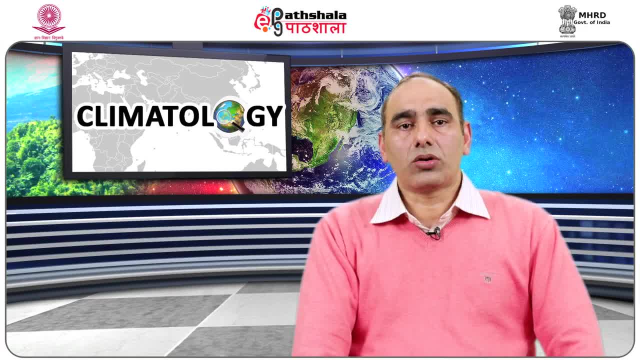 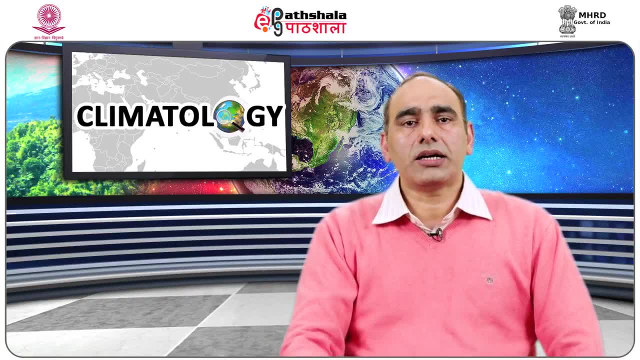 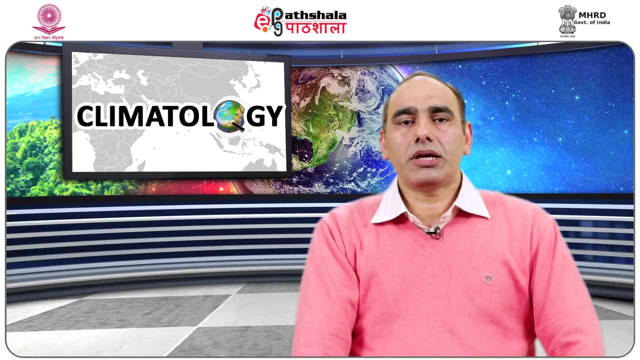 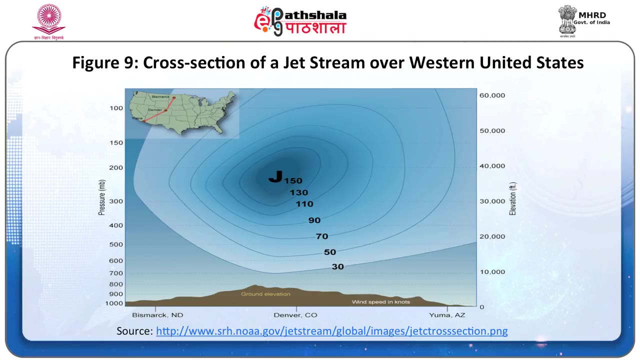 300 km per hour, According to Scholar-Nemias. A jet stream is essentially circumpolar in character, which meanders and completely gradles the Earth as upper airwesterly in both the hemispheres. Generally, jet streams are thousands of kilometers in length, about 150 to 500 kilometers wide. 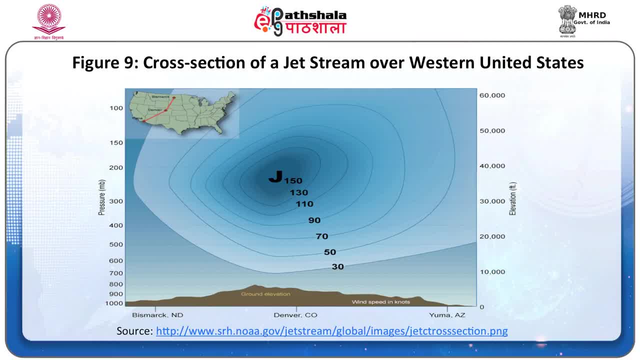 and a few kilometers thick vertically. Wind speed in jet stream is, on an average, about 140 km per hour. They move at an average speed of 110 km per hour in summer and about 190 km per hour in winter, But occasionally the wind velocities may be about 450 km per hour or slightly more. 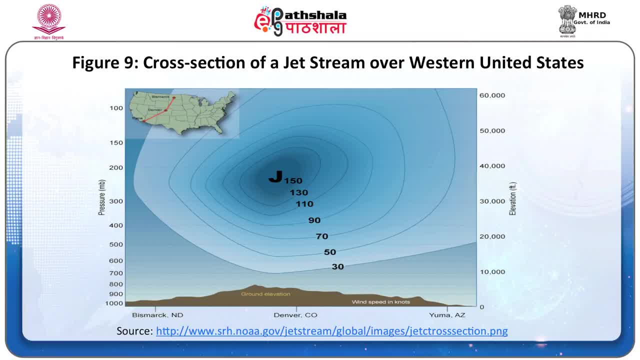 Over Northern America. wind velocity on an average in a cross section of jet stream is about 60 km per hour in summer and it around doubles to about 125 km per hour in winter. The vertical shear of wind, that is the gradient of wind velocity with height, is of the order. 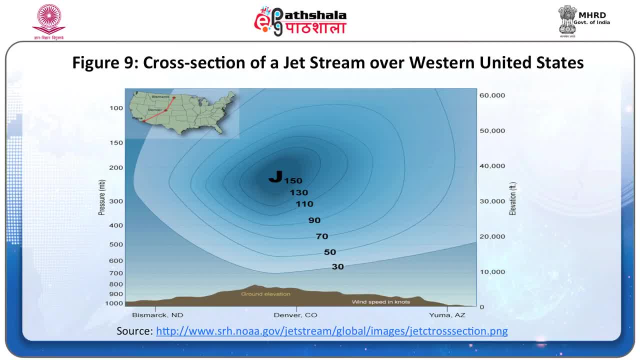 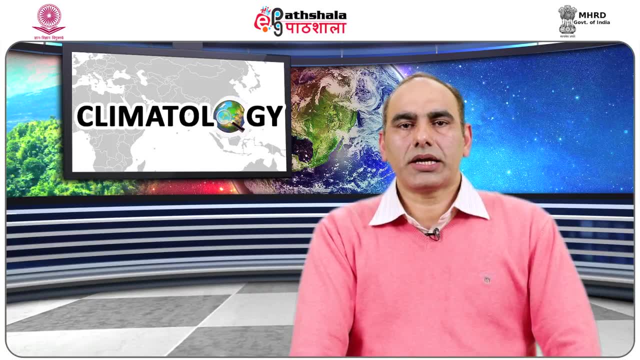 of 5 to 10 m per second per kilometer. The lateral or horizontal wind shear is about 5 m per second per kilometer. An arbitrary limit on the lower side for wind speed along the axis of a jet stream is 30 m per second. 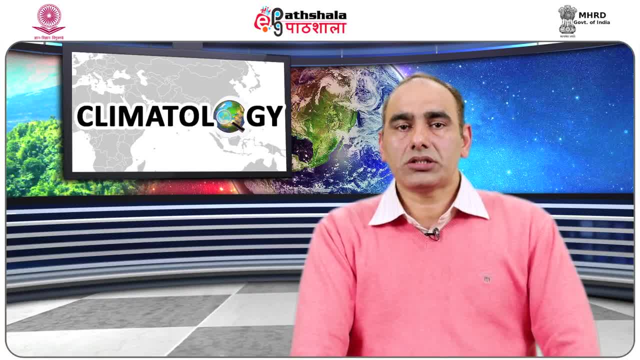 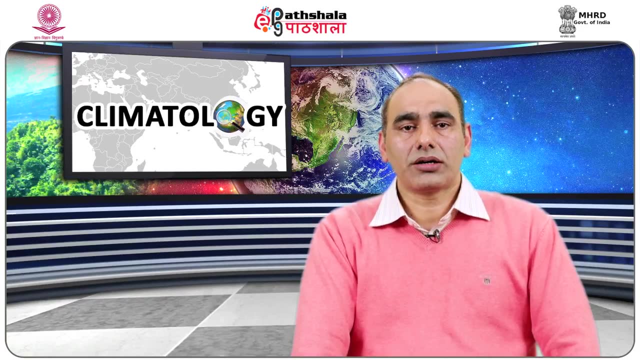 The highest velocities of jet streams are observed in its core region. Generally, as the jet moves from over an ocean to over a continent, its velocity increases due to steeper pressure gradient. Conversely, while moving from a continent to over an ocean, the velocity normally decreases. 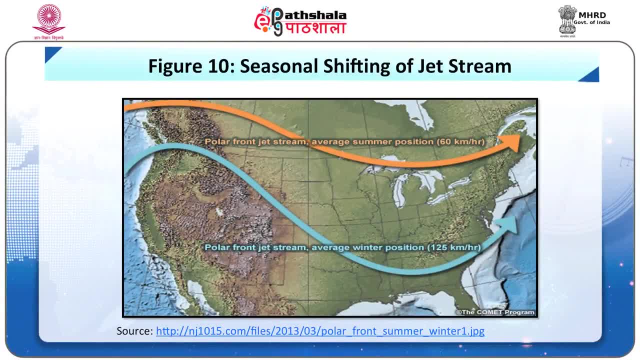 Jet streams are characterized by great seasonal shifts in positions, With a change in overhead position of sun. the jet streams shift poleward in summer and equatorward in winter, as can be seen in the figure 10.. In winter, the pressure gradient is 10 m per second per kilometer. 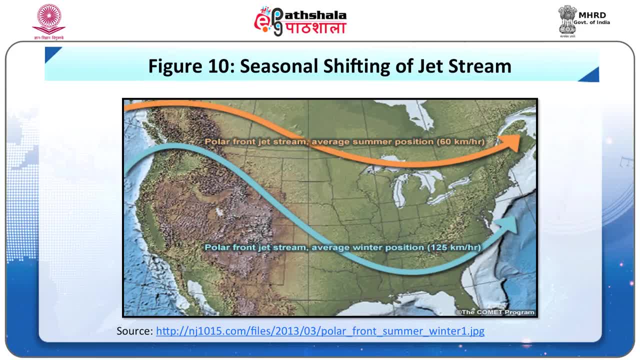 In winter, the pressure gradient is 10 m per second per kilometer. In winter, the pressure gradient is 10 m per second per kilometer. In winter, the pressure gradient is 210 m per second per kilometer. The jet streams follow meandering pathways during the summer season. 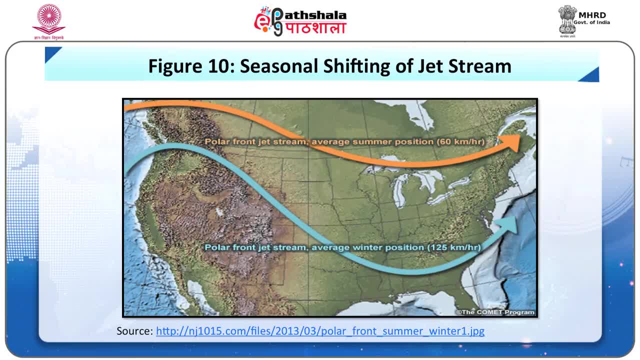 In summer season, the crest, or beasts of the roast bees, are located over the continents and the troughs over the oceans. In winter, the continents are under the troughs of the waves, the oceans are under the crests, The seasonal northward and southward shifting. 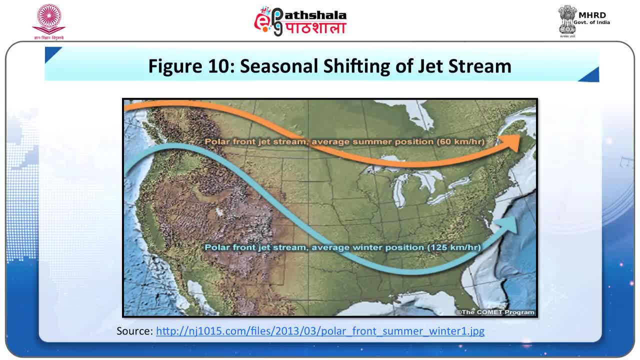 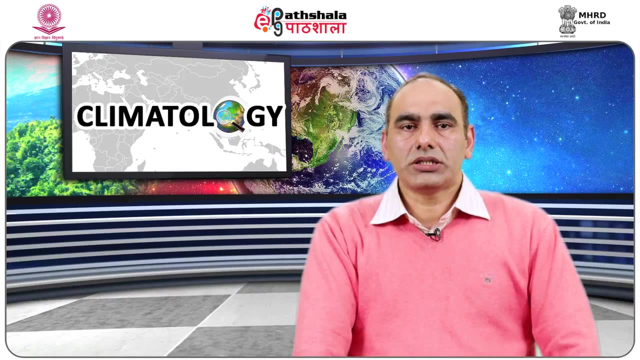 is also more conspicuous over the continents than over the oceans. This is mainly due to the differential rates of heating of land and sea. Let us come to the origin of jet streams. The origin of winds and its velocity are function of pressure differences, which are result of temperature variations. In case of 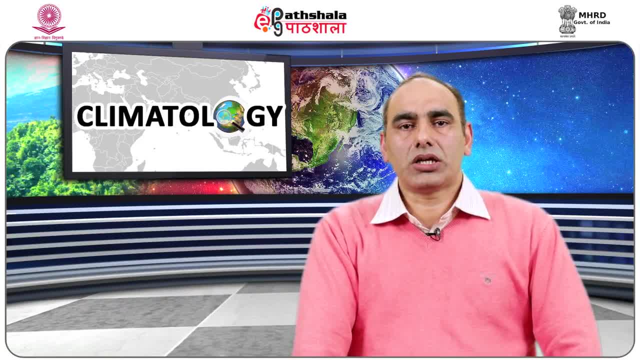 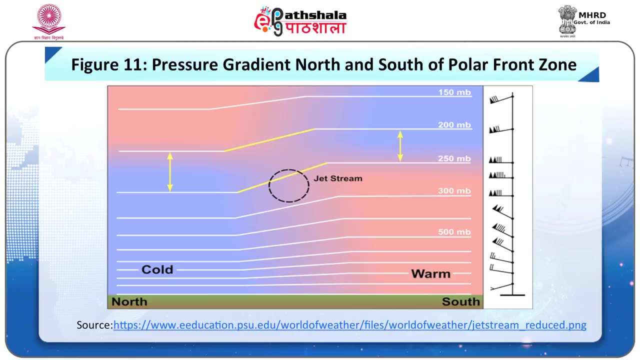 polar jet stream. this temperature variation is a result of contrasting cold air mass on polar side and warm air mass on equatorial side of the polar front zone. As cold air is dense and compact than warm air, air pressure decreases at a faster rate in colder air mass. 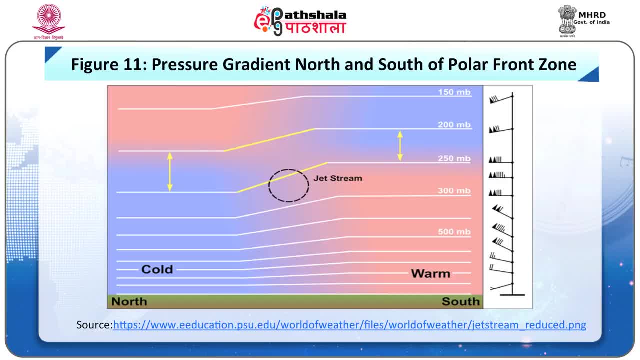 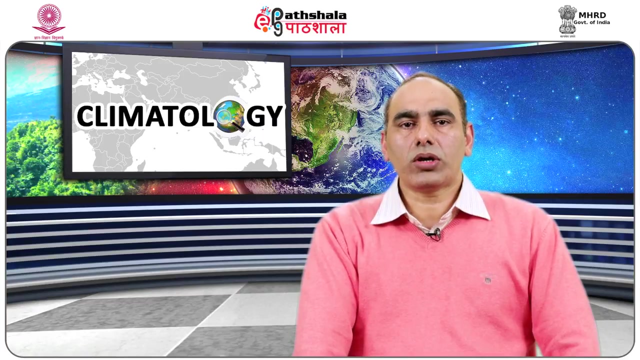 as as compared to warm air mass or column of air, It means that north of the polar front zone there is a higher pressure as compared to its south at one particular altitude. You can refer figure 11.. As a principle, temperature falls more rapidly in a warm column of air with altitude and. 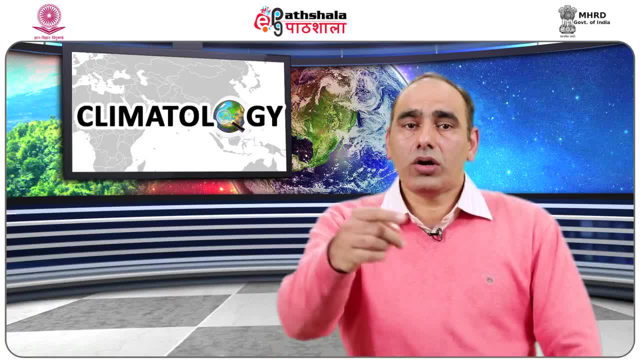 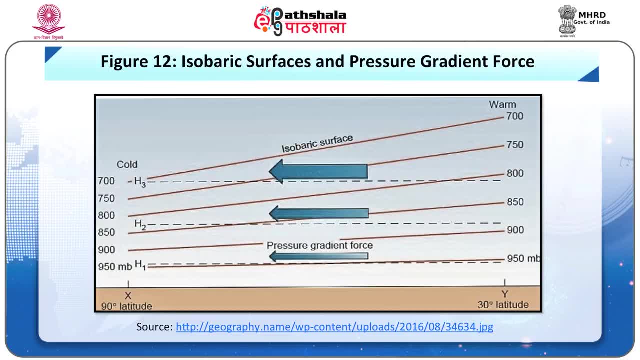 pressure falls more rapidly in a column of cold air with altitude. Thus the fall in pressure with altitude is higher in case of areas of low temperature. Therefore, the fall of pressure north of polar front is steeper than towards its south. In such a situation, an isobaric surface, ie equal pressure plane in atmosphere, will be. 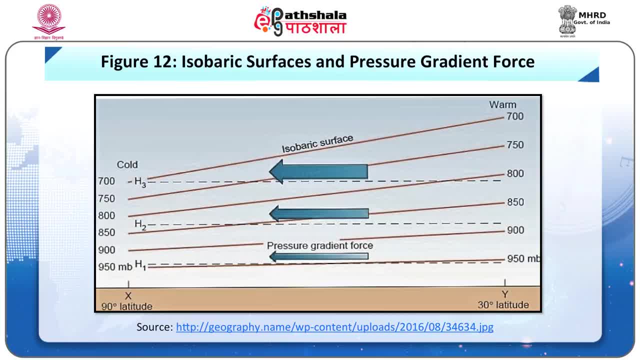 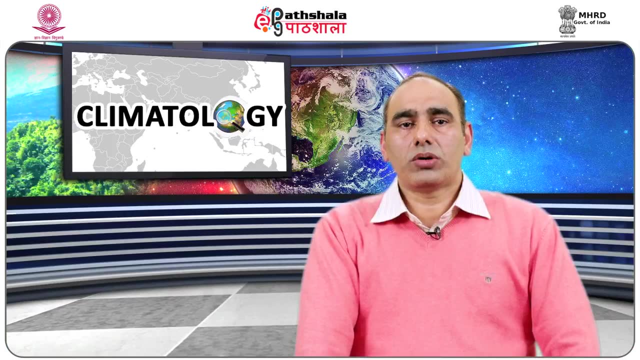 sloping towards north. Thus the fall in pressure will be steeper in case of areas of high pressure on ground. Also, the isobaric surfaces of the successively lower pressure will become steeper with higher altitudes, As can be seen in figure 12.. 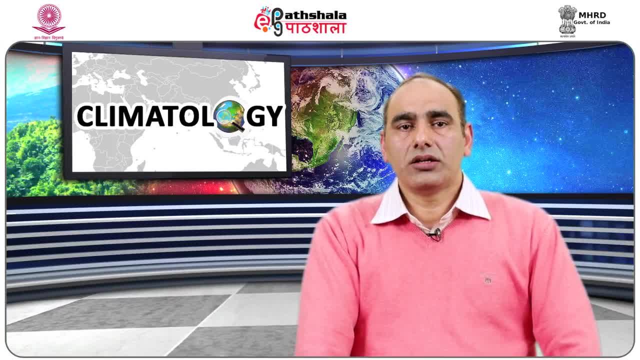 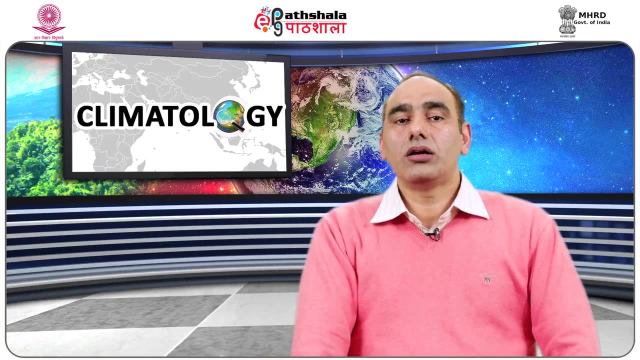 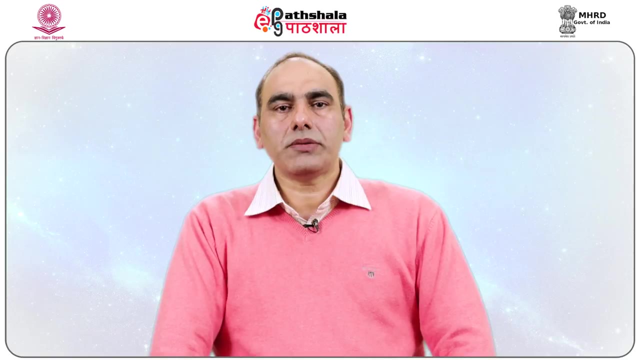 Over the tropical region. as temperatures are higher, air pressure decreases more gradually than over the cold polar areas. Consequently, at the same altitude Above the surface surface, higher pressure prevails over the tropics and lower pressure over the polar areas. Therefore, the resulting pressure gradient is directed towards. 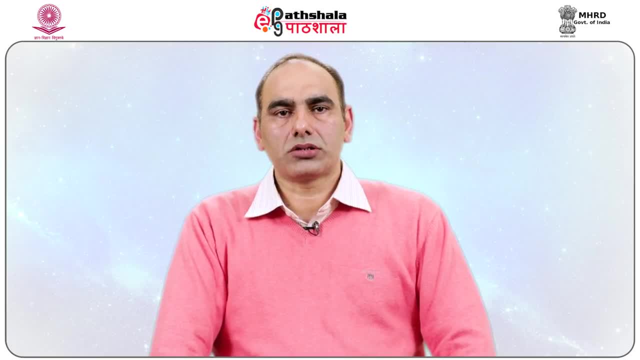 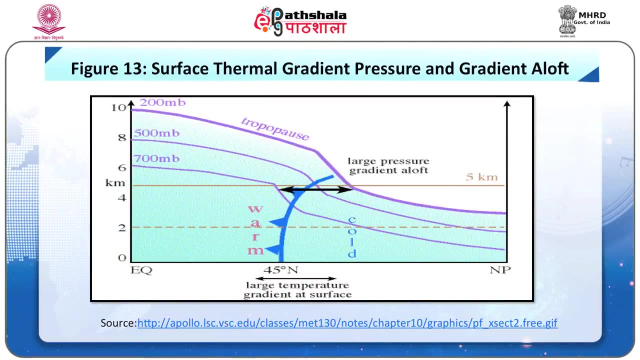 areas of high pressure, that is, tropics, towards the areas of low pressure, that is, polar areas. Thus thermal contrast at surface results into steep pressure gradient in upper air. The intensity of the thermal contrast is at peak during winter season. Therefore the pressure gradient and resultant jet streams are 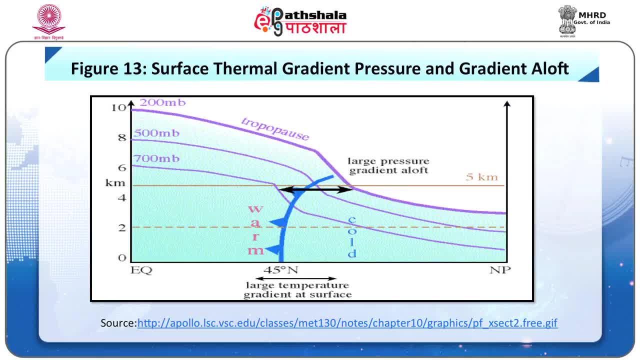 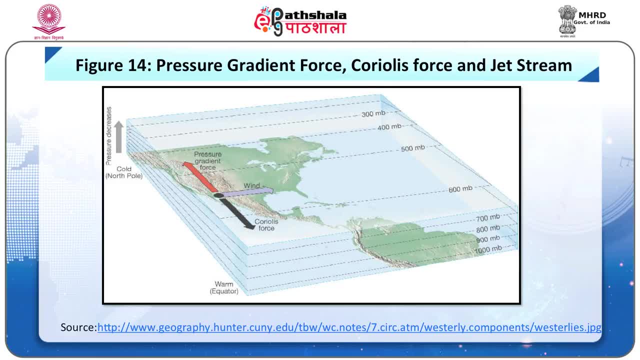 strongest during winter, as can be seen in figure 13.. Due to pressure gradient force, air motion should be from tropics to poleward, as indicated by red arrow in figure 14.. But the Coriolis force also comes into play and counterbalances the pressure. 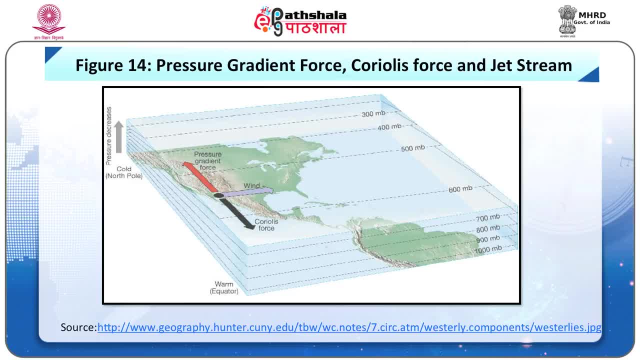 gradient force. Therefore jet streams as a geostrophic wind moves from west to east as upper air westerly. The key aspect of origin of jet stream is large thermal contrast at surface which produces steep pressure gradients aloft. Here stronger upper air winds as jet streams within the slower general westerly flow or as core of roast. 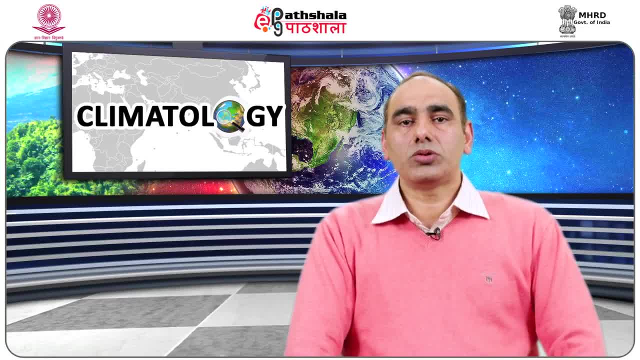 B waves develops. Let us come to types and distribution of jet streams. On the basis of their location or distribution, jet streams are classified into following types: Polar jet stream. subtropical jet stream. easterly tropical jet stream. stratosphere jet stream. 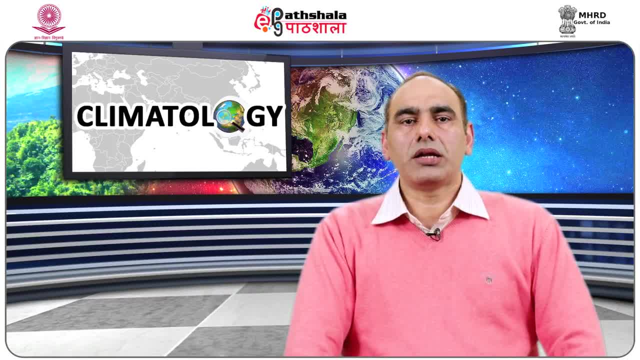 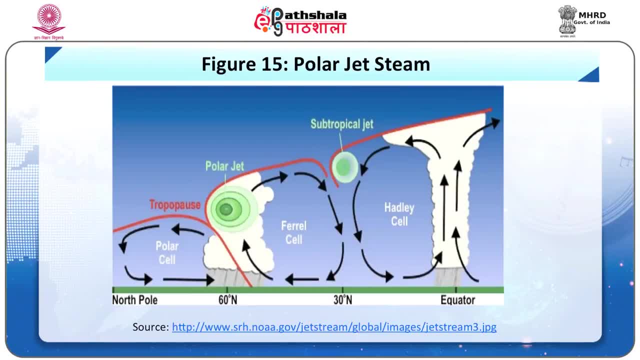 stratospheric, sub polar jet stream and, finally, local or regional jet stream. Let us discuss them one by one. First, polar jet stream. it is also known as polar front jet stream because it is associated with polar front. Polar fronts are linear zones which occur due to large thermal gradient created by convergence. 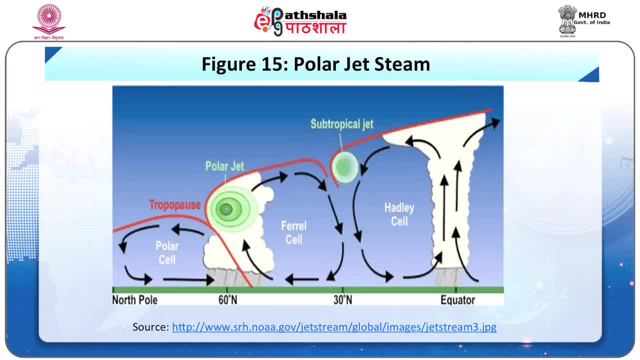 of contrasting cold air mass of polar areas and warm or mild air mass of tropical areas. It occurs near tropopause between polar cell and feral cell, as can be seen in figure number 15.. They are most active at 300 millibar, that is, at altitude of about 9 km within 40 degree. 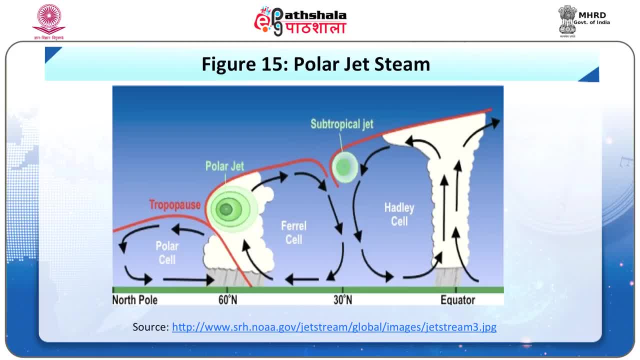 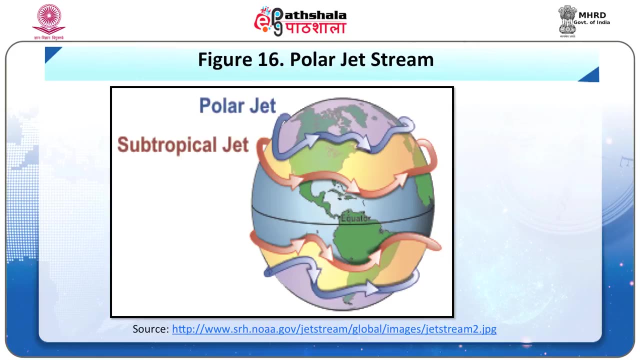 to 60 degree latitudes. The seasonal shifting is in the range of 30 to 60 degree. It is also known as subtropical westerly jet stream. It occupies a position at the tropopause between headly cell and feral cell at the altitudinal 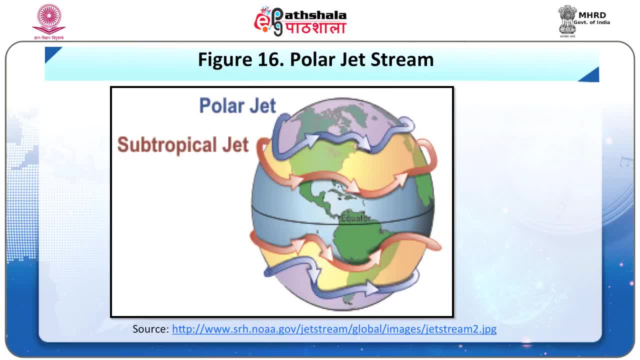 range of 9 to 13 km, as can be seen in figure number 15 and 16.. In case of this jet stream, it occupies a position at the tropopause between headly cell and feral cell, as can be seen in figure number 15 and 16.. 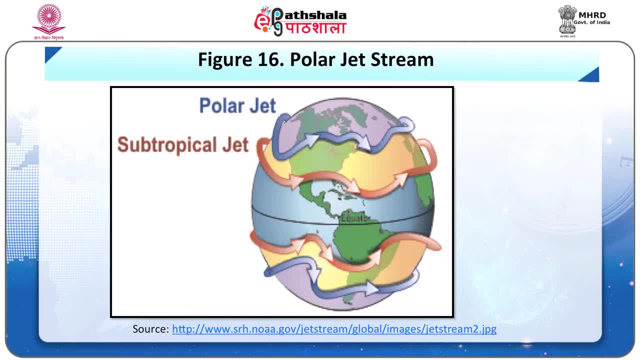 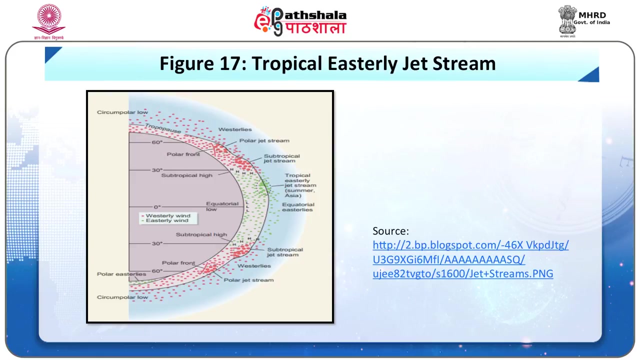 The front of contrasting air masses is not present and surface thermal gradient is also very poor. Its origin is related to a thermal gradient confined to upper tropopause. In comparison to polar front jet stream, it is much more persistent. Third one is easterly tropical jet stream. 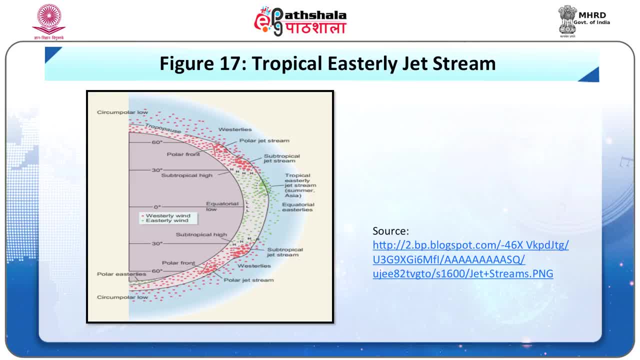 It forms in the upper troposphere over India and Africa. The horizontal region which is located in the spur of Locomotion region actually points to the northern hemisphere as well. The tropical easterly jet stream is located very high altitude, ie near the ocean. It is located about 12 km away from the垂直谷. The strong gust of wind is flip-flopping in the lower part of the climate. The pressure of the jet stream reduces the descent of the jet stream from the water to. 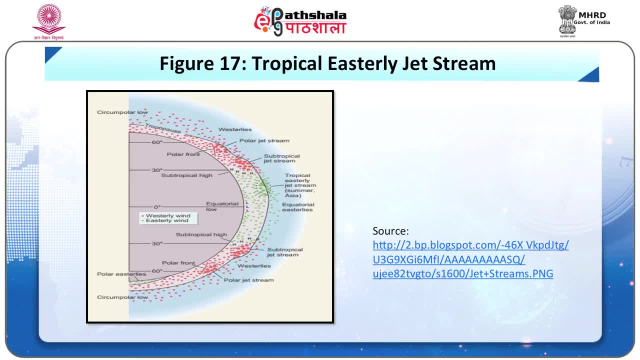 the atmosphere, which increases the temperature and the humidity. It raises the temperature and the humidity in the air. It is about 8 to 10 km above sea level, as can be seen in figure number 15.. It is also known as subtropical westerly jet stream. 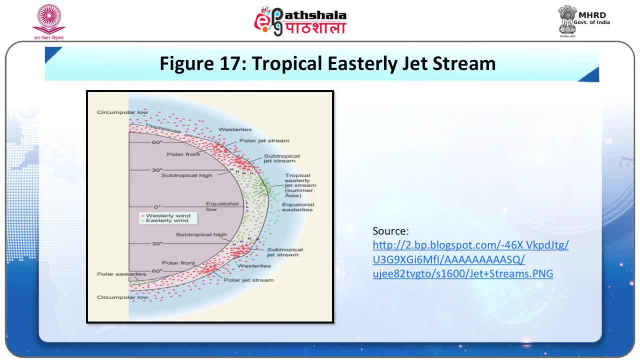 It is also very common in the southern hemisphere. It is also very common in the southern hemisphere. The tropical easterly jet stream takes up the water depth between head to the ocean. only this jet stream occupies position at very high altitude, that is about 15. 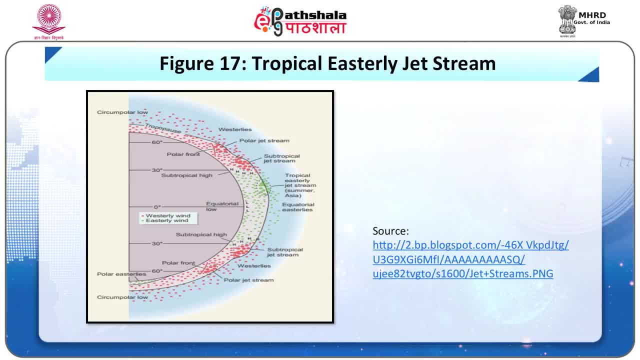 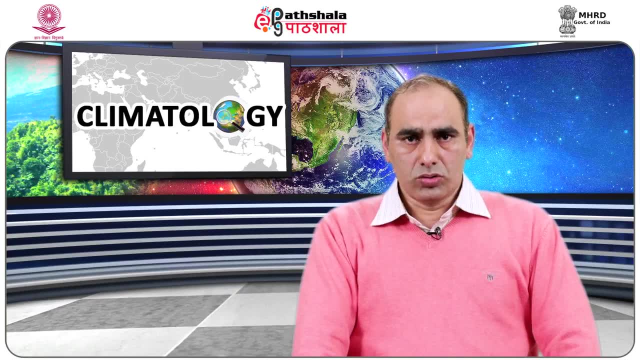 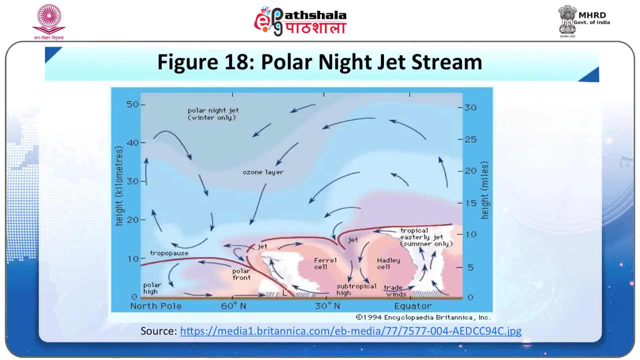 kilometer. it is located over the headless cell, as can be seen in figure number 17. it plays a significant role in monsoon mechanism. the extent of monsoon season in Southeast Asia is associated with its presence. fourth one is stratospheric subpolar jet stream. these are also known as polar night jet. 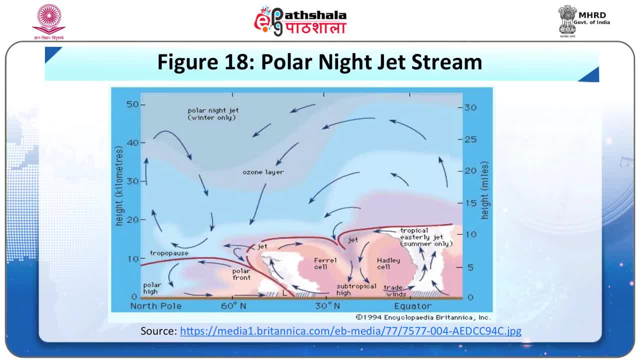 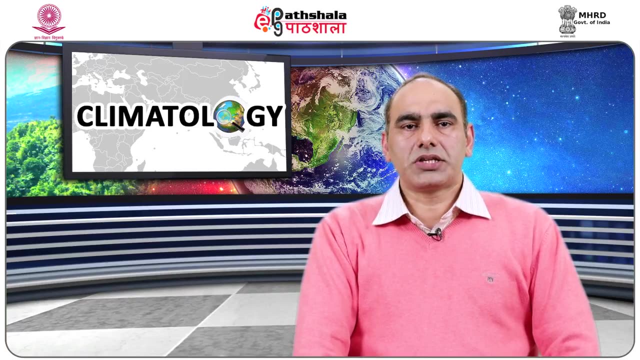 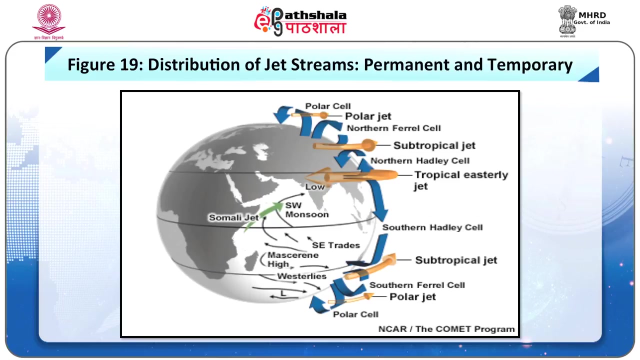 streams. they originate in stratosphere at an altitude of about 30 kilometer around the poles in winter season, as can be seen in figure 18. finally, local or regional jet streams: over the period of time, due to better data acquisition techniques, and scholars have identified many local or regional jet streams of temporary nature. 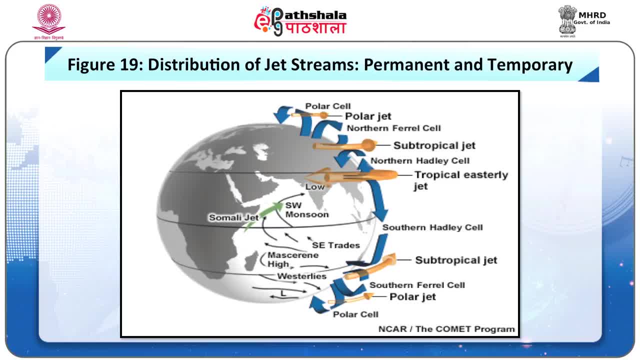 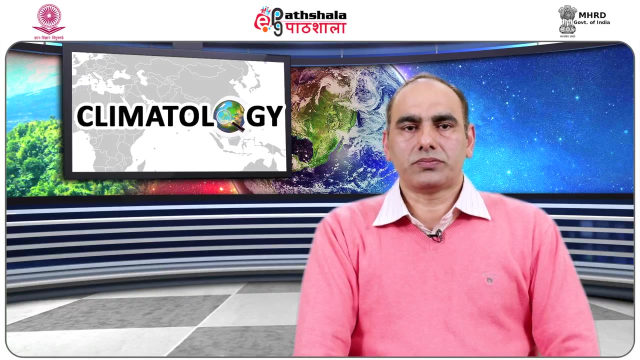 for instance, Somali jet stream, which can be seen in figure 19. they originate due to local level, thermal contrast and dynamic changes in upper troposphere. these have significance in influencing local weather conditions. let us now come to the significance of jet stream. although weather scientists are not yet fully aware about the origin, forms and 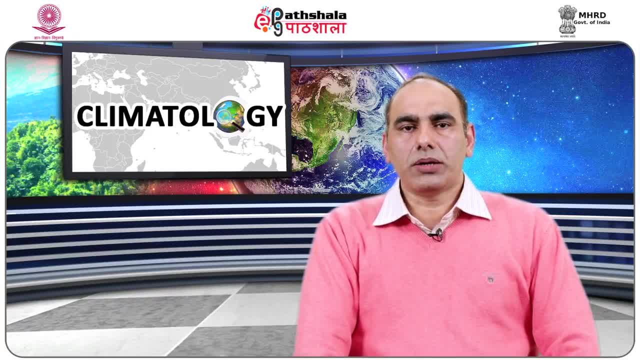 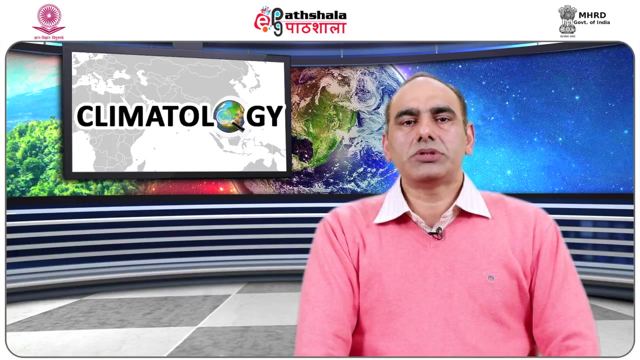 features of different types of jet streams, yet they have been able to establish relationship of jet stream with many surface weather phenomena. the most well understood and well established relationship is between jet streams and mid latitude temperate cyclones. in the belt of western west lease, the troughs and ridges of Rossby, waves and jet streams are associated with. 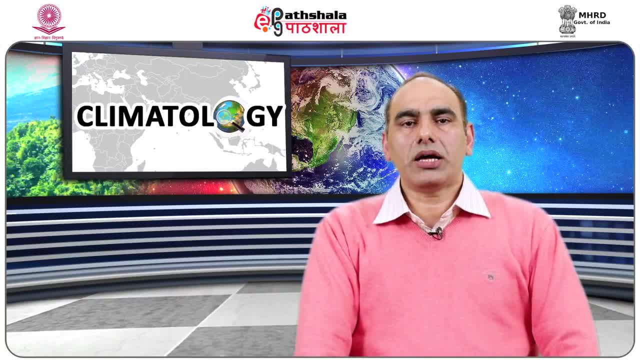 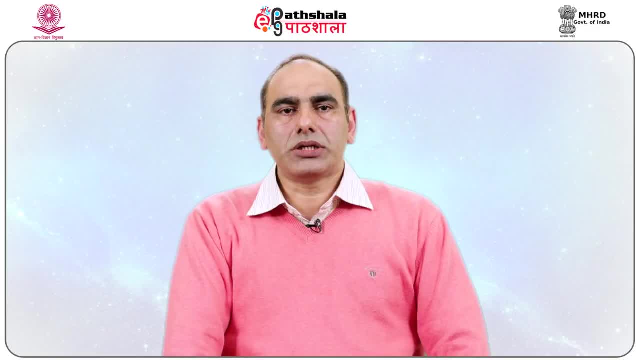 cyclonic identity. cyclone in conditions in the upper air as well as on surface, temperate cyclones and SECA, associated precipitation is about normal whenever a prayer, that seems our position over cyclones. the index cycle of jet streams resorts into latitudinal heat transfer between tropic and or. 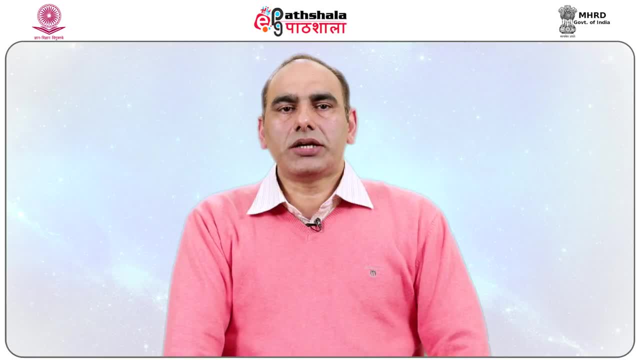 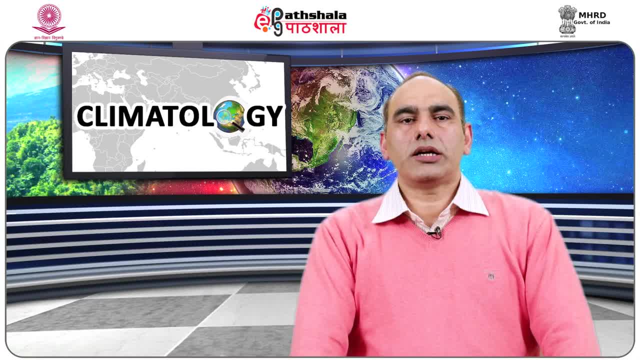 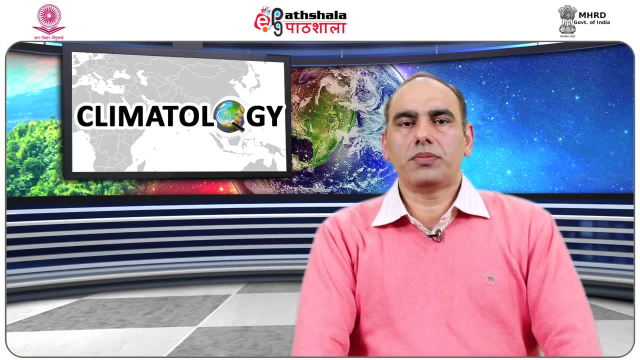 the great plains of India in winter season. Till the time jet stream prevails over this area, it maintains a pressure gradient from north to south and this is not in favor of onset of southwest monsoon over India. Therefore, the shifting of subtropical jet stream north of 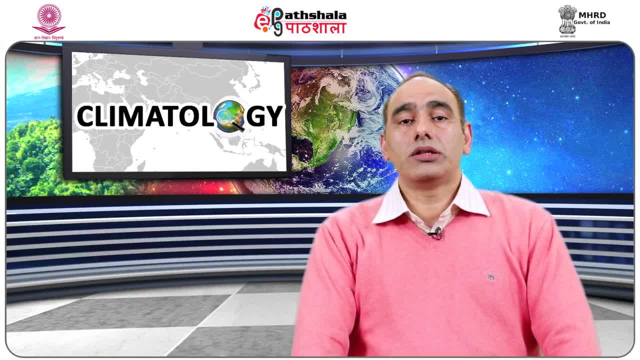 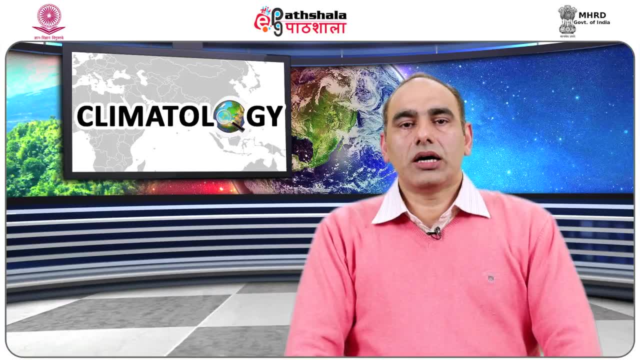 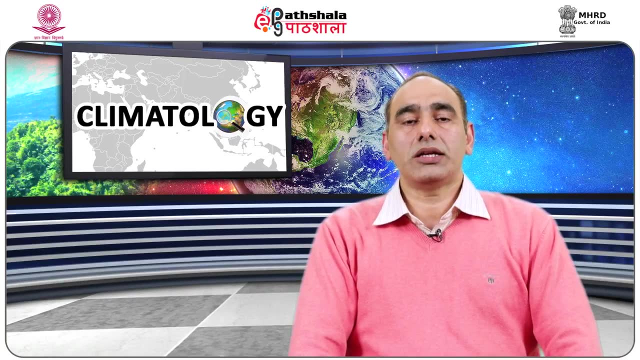 Himalayas is prerequisite for the establishment of headly cell over Indian subcontinent In summer season. the temporary tropical easterly jet stream also plays significant role in monsoon mechanism. The jet stream plays a very significant role in monsoon mechanism because it tends to strengthen the summer monsoon. 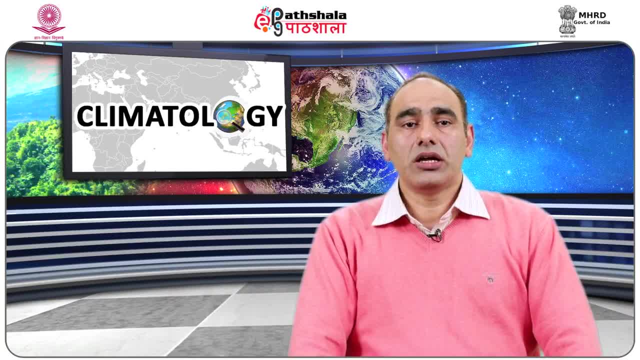 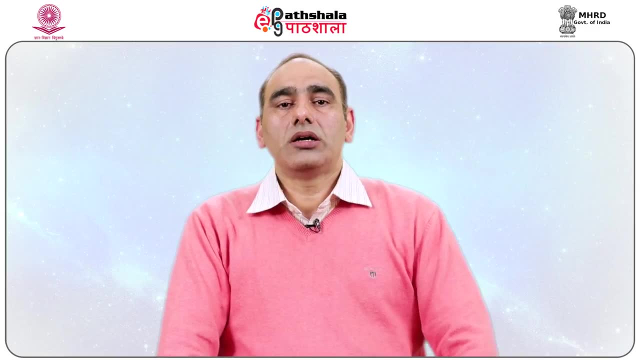 Subsiding air on its left margin creates a high pressure over the Bay of Bengal and the Indian Ocean, while rising air under its right margin causes low pressure under its right margin over the Great Plains region. therefore, it helps in enhancing the south專tial hot water Earlier mentioned combine between south and north Nationalпар obituaries. 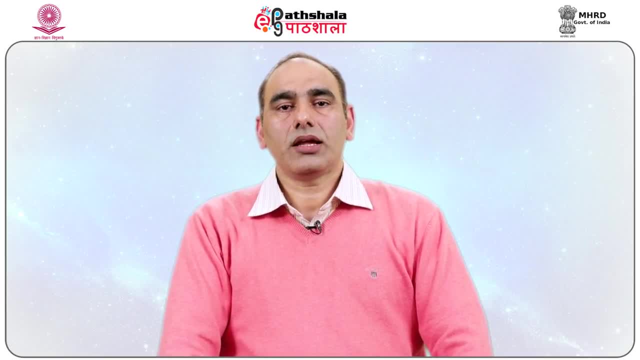 to north pressure gradient steeper. Hence it is associated with the strength and length or duration of southwest monsoon season. Subtropical westerly jet streams bring western disturbances in northwest India during winter season. This results in precipitation in North India during winter season Jet streams. 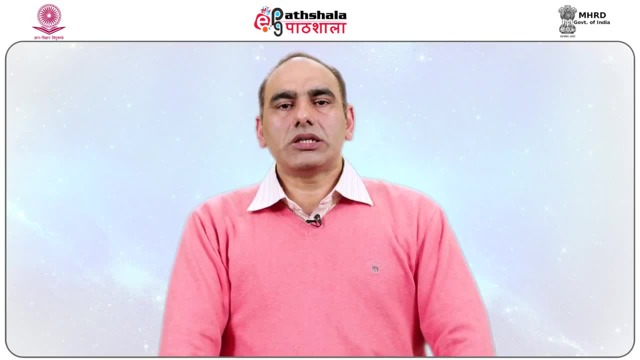 also play an important role in the movement of air masses and associated weather changes in the trajectory. Thus, it is well established that jet streams play a significant role in surface weather phenomena. Let us come to the summary and conclusions: Temperature, atmospheric pressure and air. 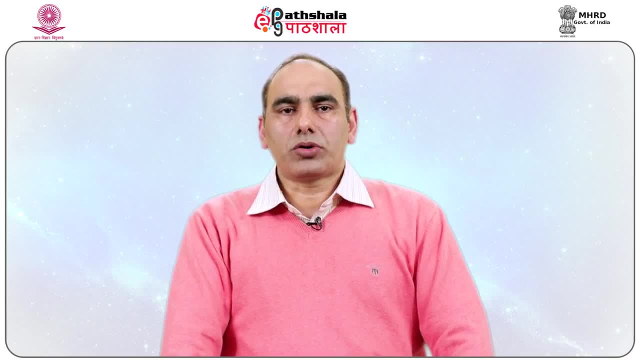 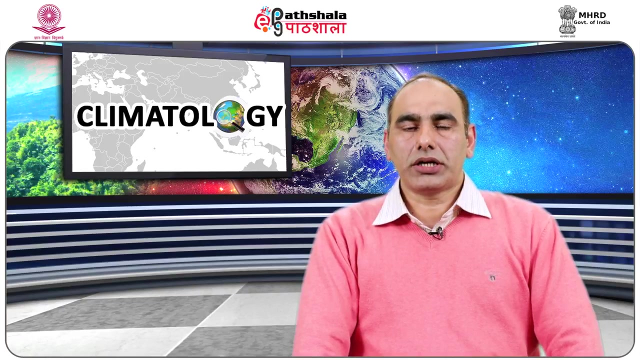 circulations are quite different. Temperature in the upper part of troposphere is different from those prevailing near the Earth's surface. In the middle and higher latitudes of both hemispheres, upper air westerlies prevail due to the balancing act of pressure, gradient force and Coriolis force.